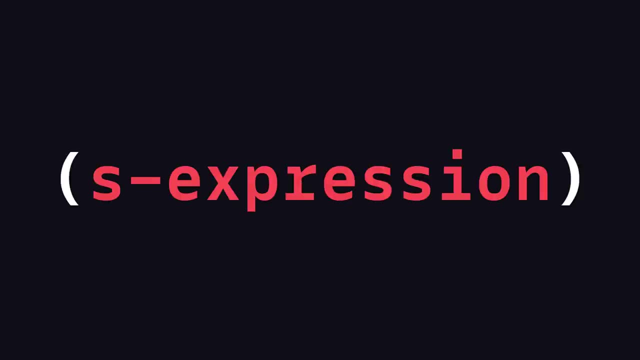 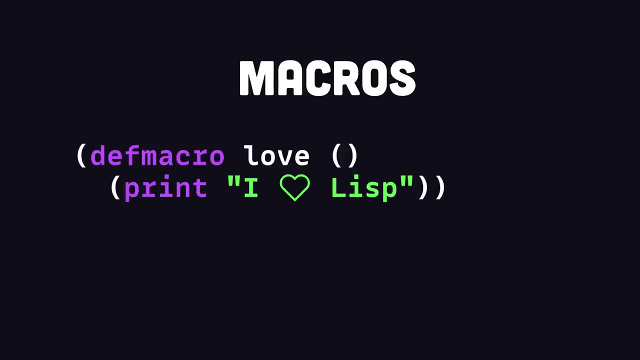 points to the next element in the list. Developers write S-expressions which might start with a function or operator, followed by one or more arguments. This gives rise to a powerful macros feature where developers can extend the syntax of Lisp and create domain-specific languages. 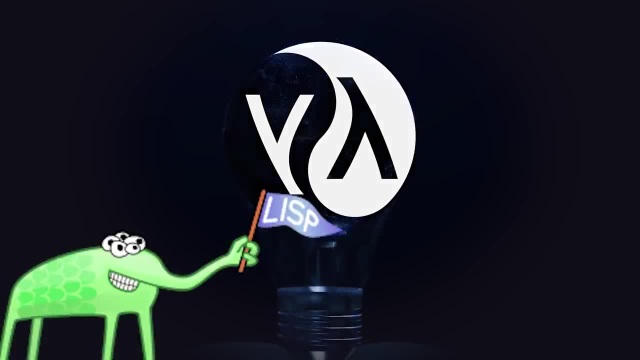 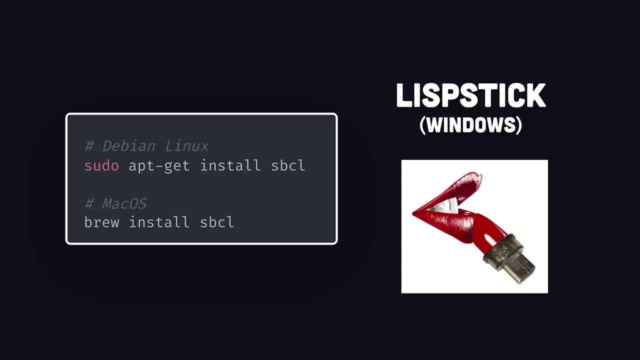 It's like a programmable programming language. Common Lisp is still in use today, but it's directly inspired many other languages like Scheme, Clojure, Ruby and JavaScript, just to name a few. To get started, install Common Lisp on your machine, then create a file ending in lsp. 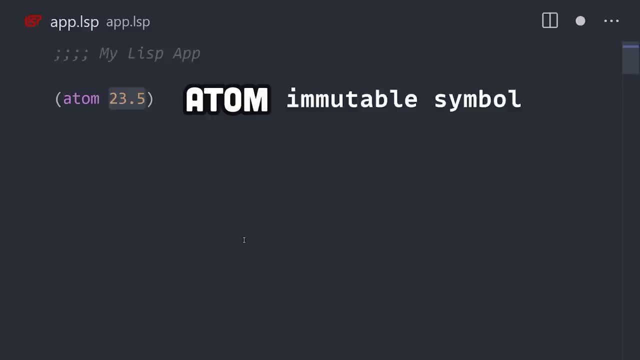 First create an S-expression which can represent an atom like a number or symbol or a list of multiple values To print to the standard output. we can reference the format function followed by T for true, then the string we want to print out, And it contains a ton of built-in functions like 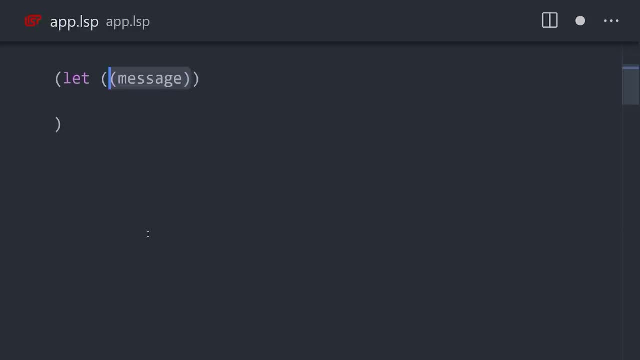 int. to simplify things, Define a local variable with the let keyword and it will be lexically scoped to the context in which it's defined. However, you can also define global variables with defparameter or defvar, which are dynamically scoped and can be used anywhere. All these 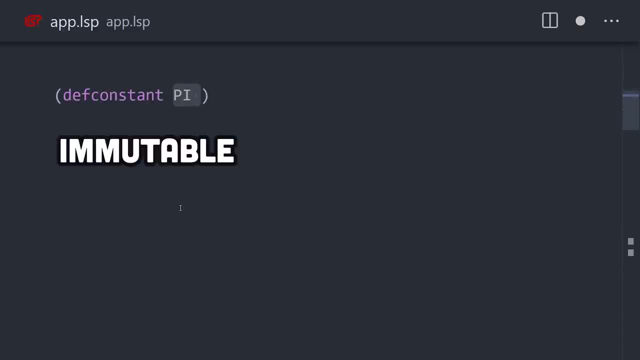 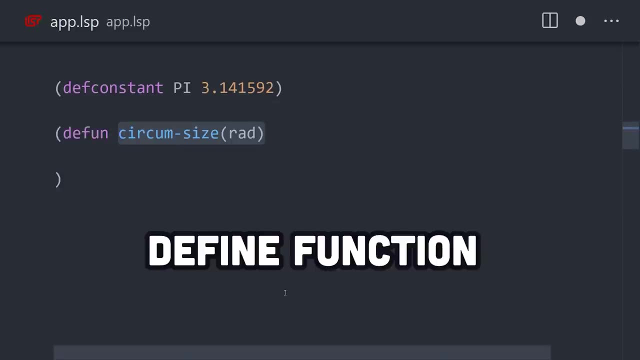 variables can be modified. however, you can also create immutable data with defconstant. Lisp is multi-paradigm but most well-known as a functional language. Use the defunkeyword, which is definitely the way you pronounce it, to define a function. It can take one or more parameters and is 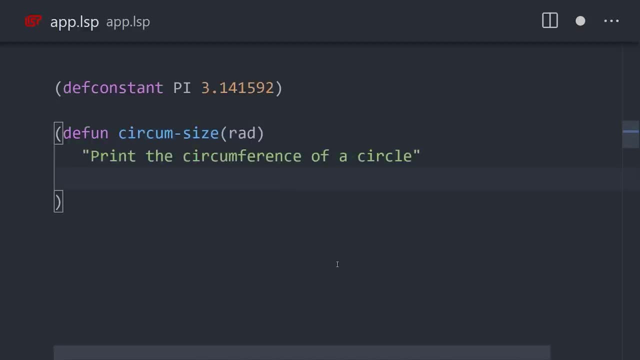 optionally followed by a string to define its purpose. You can use the star operator to multiply pi by the input radius, and the last expression in the function body will automatically be used as the return value. It was the first language to support higher-order functions where we might do something like create a list, then use another function. 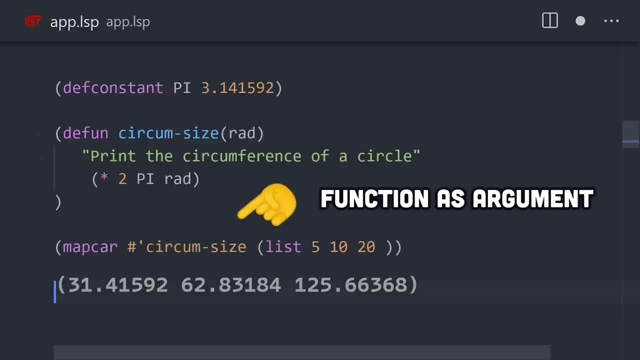 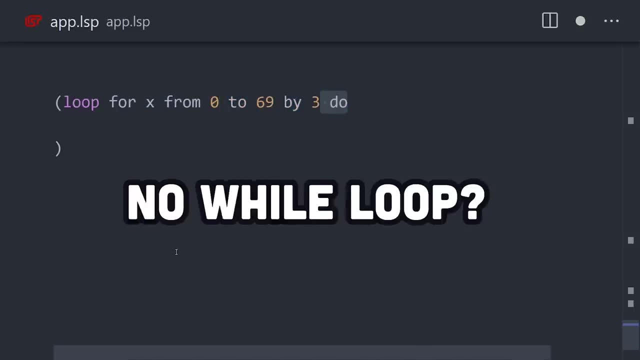 called mapcar, to loop over that list and call the function we just defined on every single element inside of it. It also includes a built-in macro called loop for general-purpose iteration. What it doesn't have, though, is a while loop. Not a problem, though, if you want to create one. 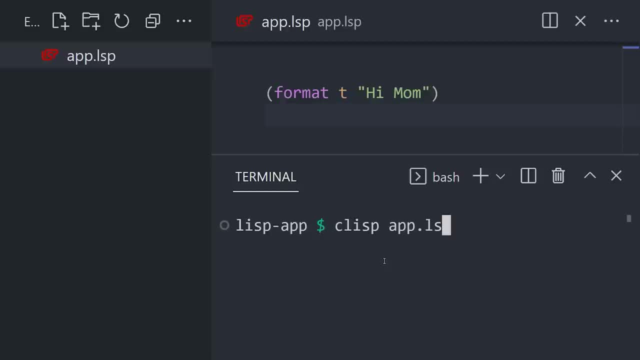 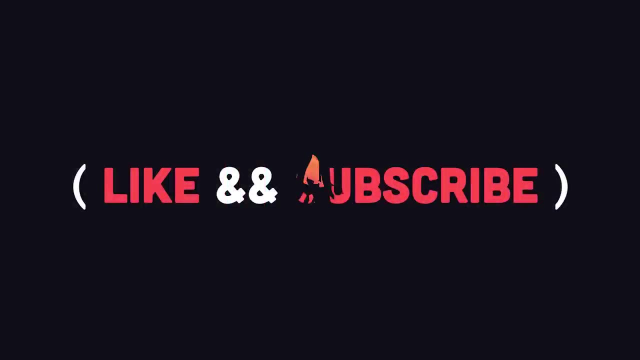 just write your own macro to extend the language. This has been Lisp in 100 seconds. Hit the like button if you want to see more short videos like this. Thanks for watching and I will see you in the next one.